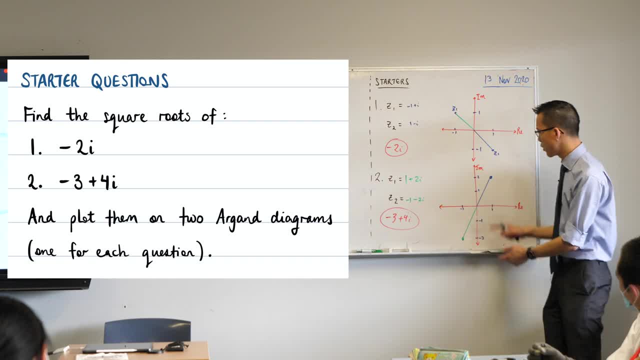 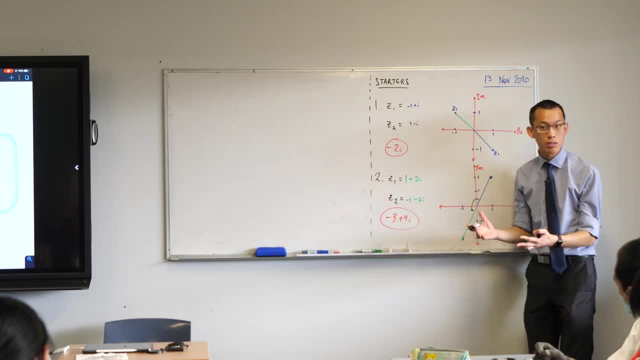 happening. just from the quadratic formula, Does that seem familiar? So you've got these kind of when you have a look at the arguments, a 180 degree or a pi radians difference between them. The other thing that I think is helpful- and I asked some of you to do this, but not all of you, so maybe, if you haven't done this already, 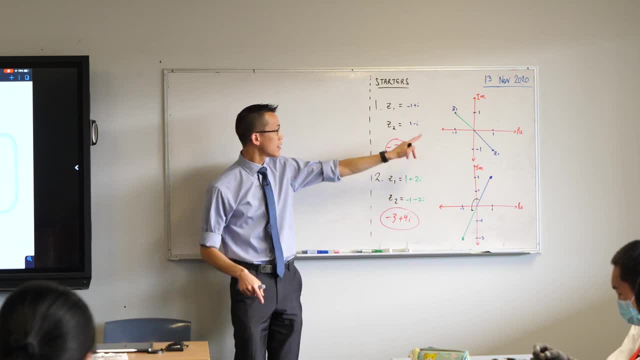 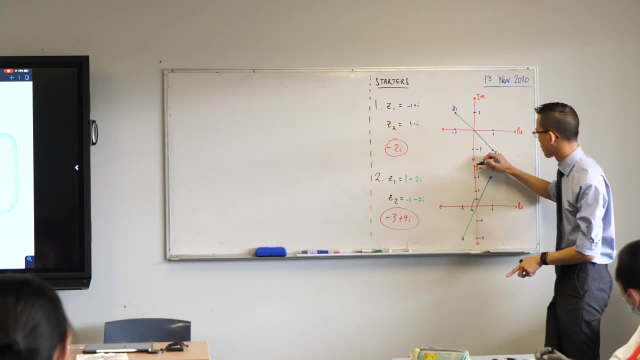 go and have a look at your first diagram right now. If you've got space, go ahead and put the actual number, the number we found the square roots of, put it onto your R-game diagram. I reckon I can squeeze it sort of. this. one is down here on this scheme. that's minus 2i. 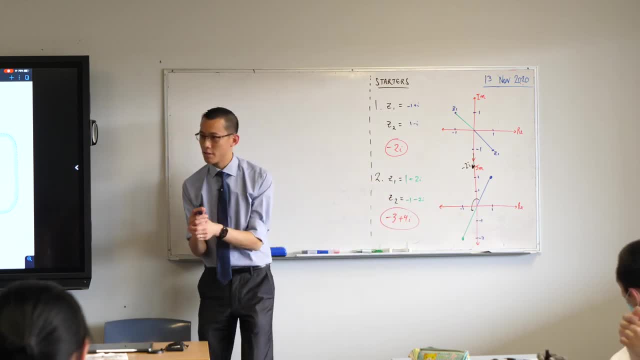 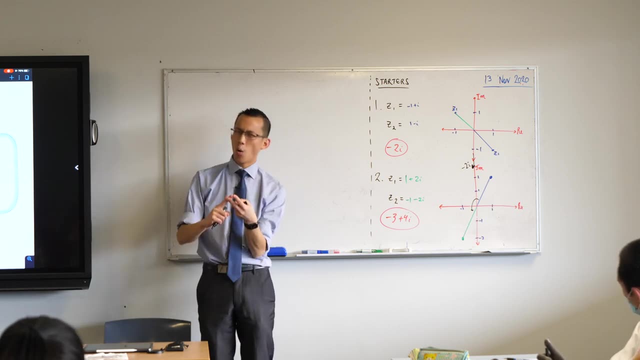 When I think about my two square roots, I think about them. I've got two ways to think about them. Number one: you can think of it as there's a clockwise square root and an anti-clockwise square root. Or you can think of it as there's a short one and a long one. There's one that gets. 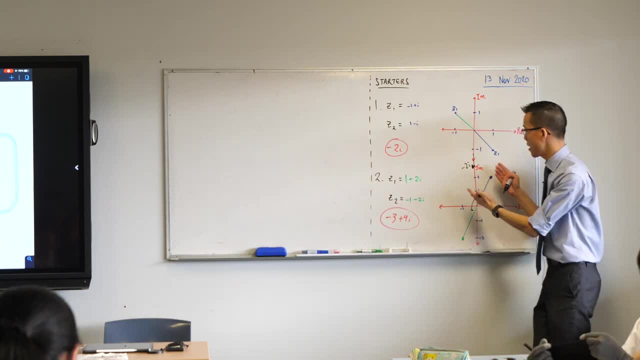 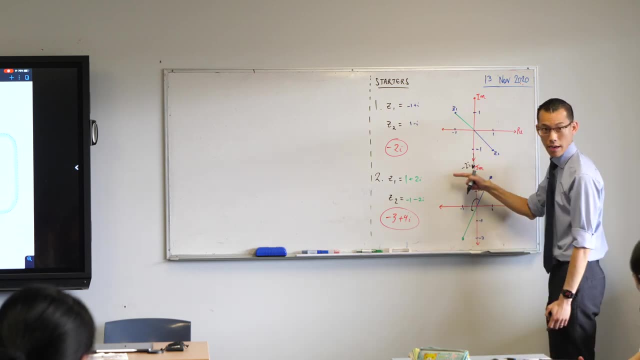 there quicker and one that gets there longer. You can see which is which when I describe it that way. To get to minus 2i in the most the laziest way, it's going clockwise. So therefore you could go negative pi on four radians, and then another negative pi on four radians And of course 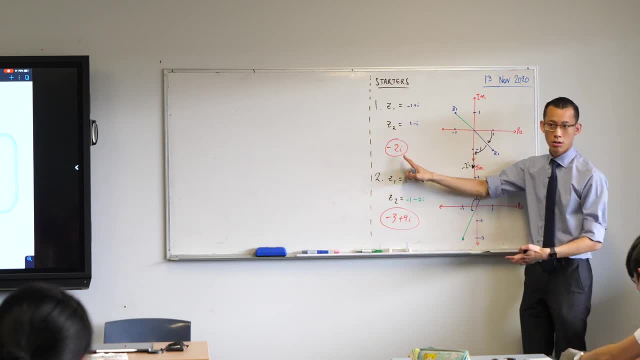 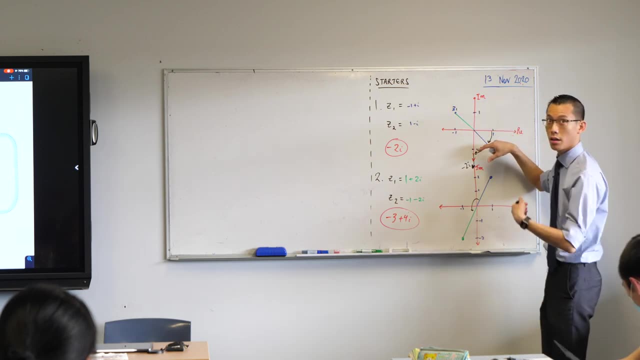 you also have the scaling. What's the modulus of our original complex Number one? it's two distance from the origin And so, as a consequence, the modulus of your square roots is going to be the square root of two, because you need to scale and then scale again. 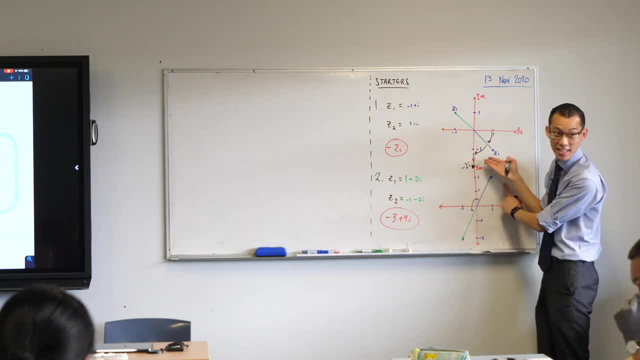 to get to your result, right? So the fast way for this particular number is clockwise, And then there's the long way, right, If you go from the positive real axis and go around that way. what's the argument of in this way, in this scheme, z1?? What's its principal argument? 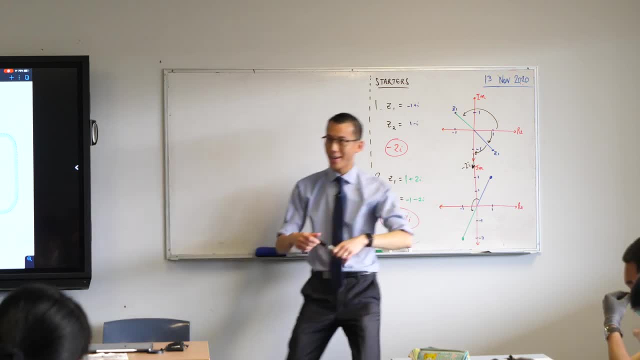 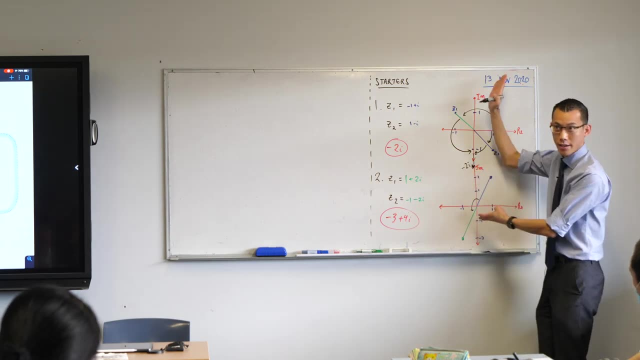 Three, yeah, three over four. pi three, pi on four. You can see if I went anti-clockwise and went another three pi on four, of course, well, actually I should be down here, but of course you still get to the negative imaginary axis. 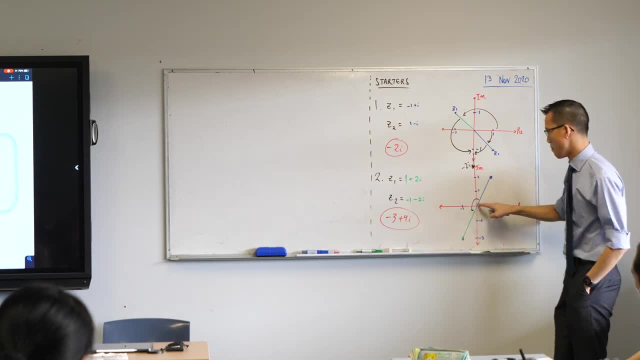 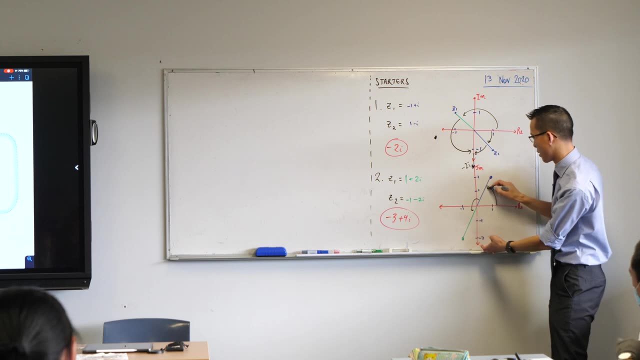 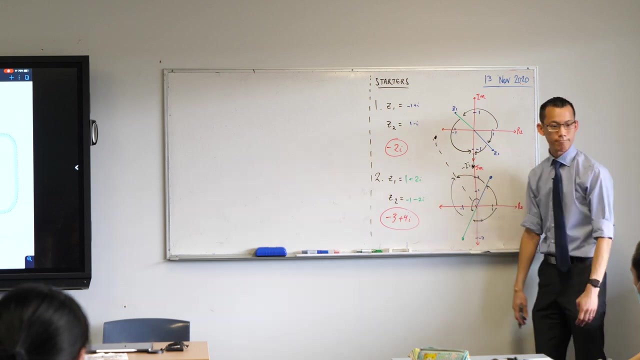 So it's a long way around- is clockwise. You can see the same thing for here. Minus three plus four, i will be somewhere up here. In this particular one, the fastest way is going anti-clockwise in that direction. Or you could go anti-clockwise like so: Sorry, that was anti-clockwise the first. 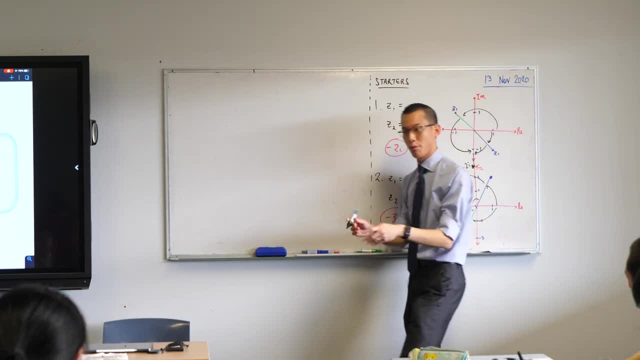 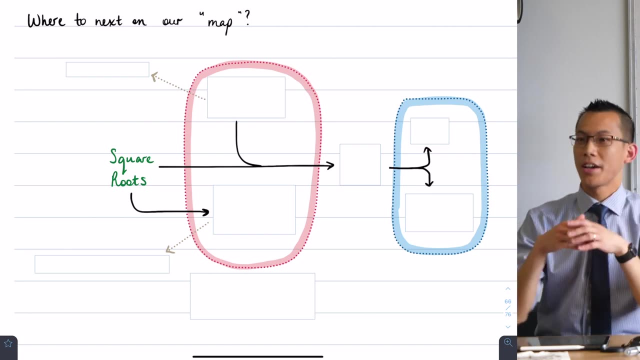 time Clockwise the second time. all right, Okay, now rule of where that is done. in case you haven't already, And if you want to start drawing this, that'd be great. As I said, we're going to move from this idea of square roots into quite a few different interconnected concepts. 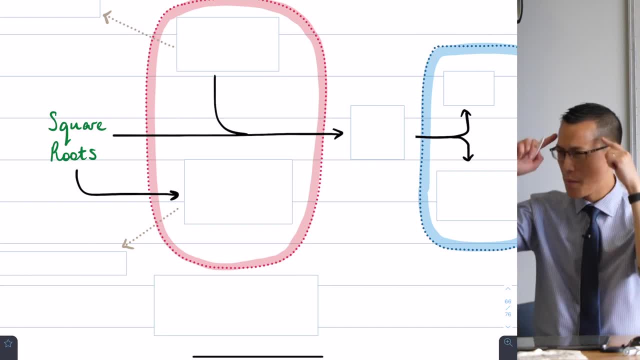 Now for those of you who are following along at home. for me, the most natural next step is we've looked at square roots, but they are not the only kinds of roots that numbers can have. For example, you could say that the- I'm trying to think of a good one- actually Square and a cube. 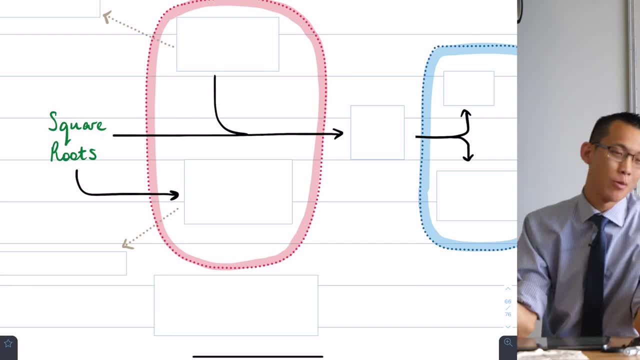 A trained professional would have thought of one beforehand. You could say: the square root of 81 is 9, right. You can say the square root of that is 9.. But you can also say that for nice numbers, the fourth root of 81, the number that you multiply by itself four times, is 3, right. 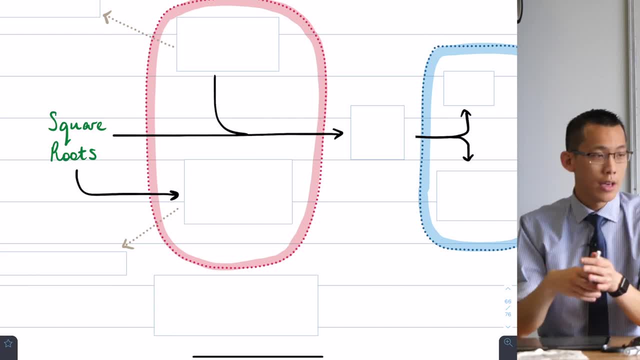 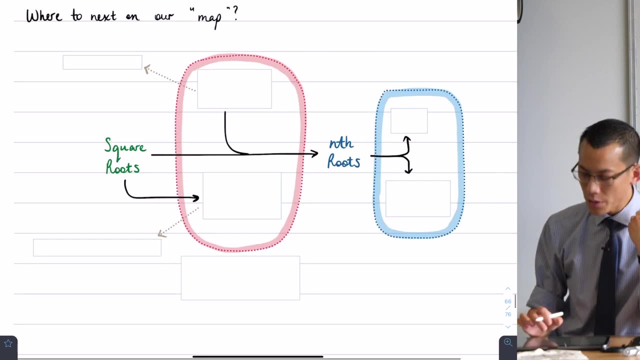 3 times 3 times 3 times 3 will give you 81, do you agree? So there's square roots- that was a fourth root example- cube roots and on and on and on. So, generally speaking, we call these guys. 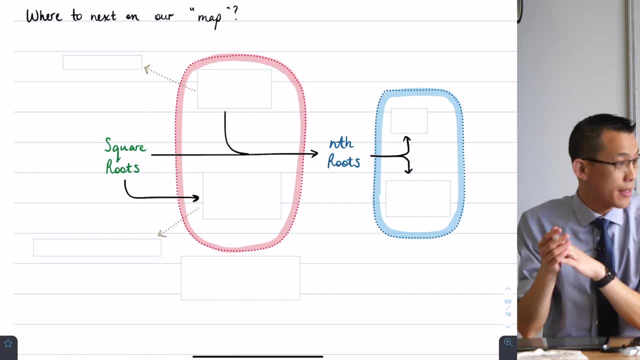 nth roots, because it can be to any degree or any power that you like. So it's a natural transition to go from square roots, which are like the special one that we deal a lot with, to this general case. okay, But it turns out as you can sort of see from the diagram, in order to get there, 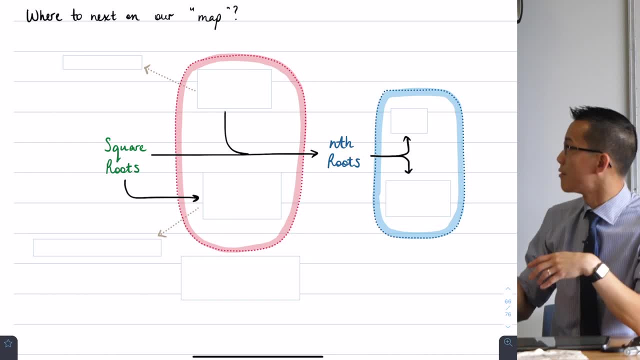 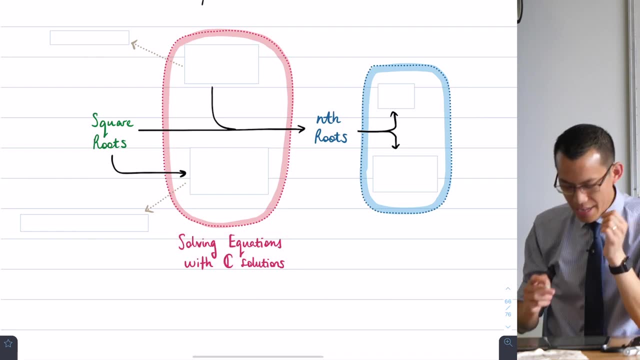 there's some other knowledge that we need another sort of building block, like you'll try and solve an equation that gets out of this and you won't be able to do it right, And that's because we need to have a solution. So we're going to be talking about solving all kinds of equations that end up. 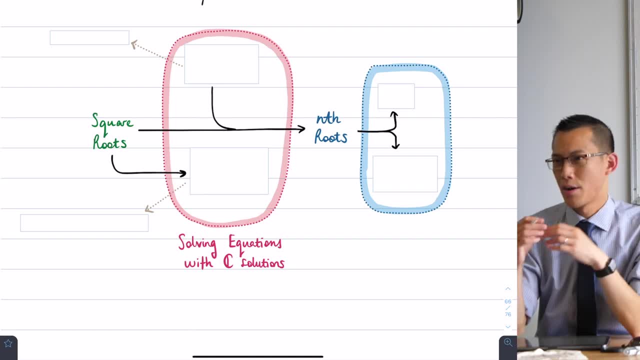 with complex solutions. Now, we actually could have done this much earlier on, but I wanted there to be a justification. I wanted it to be: you know, we're not just solving equations because we can. we're going to solve them because it's a bridge skill. to get to something else I want to do: 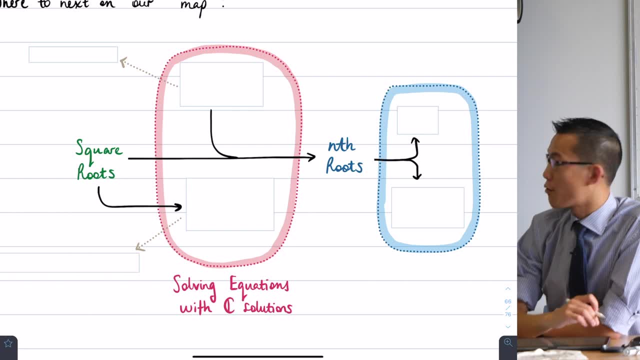 right, But there's two of them. So from square roots, right. if we combine that with solving equations which have real coefficients, we're going to be able to solve complex solutions. It'll be those two skills together that you'll find next week. allow us to solve nth roots, But now that we know about square roots, there's 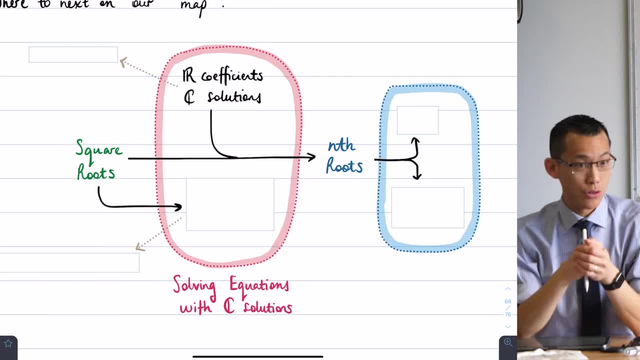 actually another kind of equation- and we're going to deal with both of these today- that you can also solve, And that is not when you have real coefficients that lead to complex solutions. but we can actually make the coefficients of our x's and our z's. we can make those complex as well. 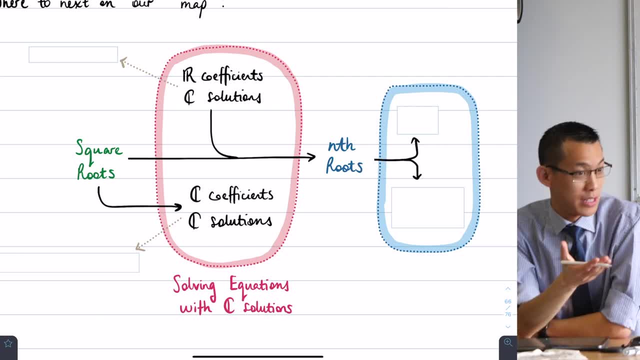 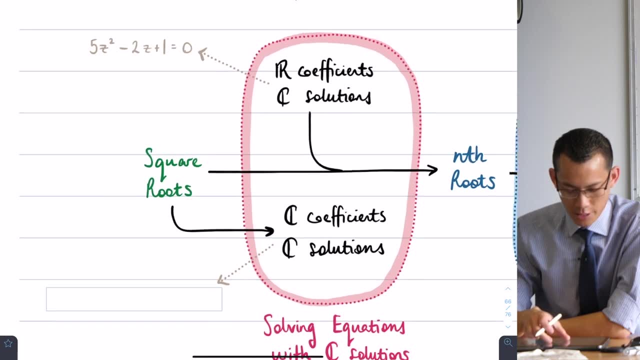 Now this is like very notation heavy, so it probably makes more sense if I give you an example, and we're going to do both of these together. This is an example of an equation. Let me make it a bit bigger for you All. the 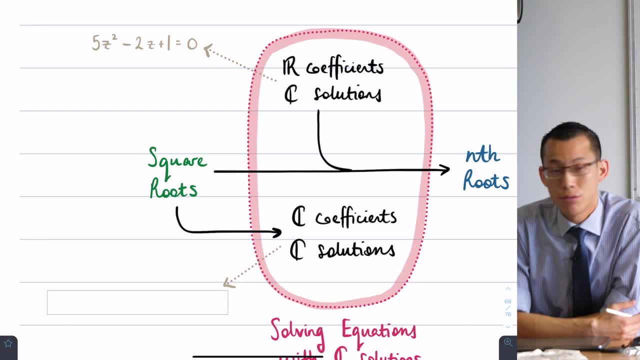 coefficients are real. Can you see that 5 and negative, 2 and 1, just real numbers? okay, But when we go ahead and solve this, we're going to find that the solutions are complex. okay, And maybe if you're having a look at this, thinking about what the discriminant will be, you'll see. 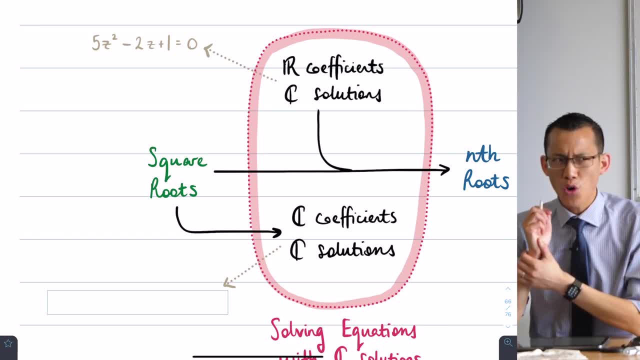 why? okay, What does an equation look like when it has complex coefficients? Well, the whole idea is: instead of numbers like 5 and negative 2, we're going to find that the solutions are complex. 2 and 1, we put in things with imaginary units and real units together, This is going to look a 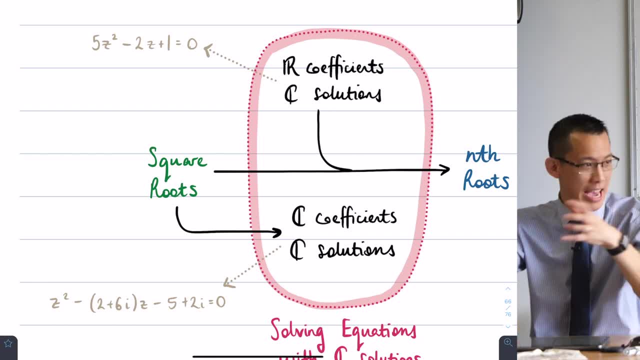 bit messier, because complex numbers are a bit messier. They have these different components to them. But you can see again. well, our a here will be 1, our b will be negative outside of 2 plus 6i. and then our c, our third coefficient. there our constant will be minus 5 plus 2i. So you can. 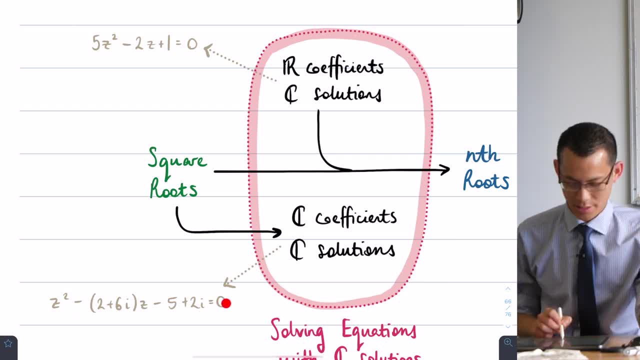 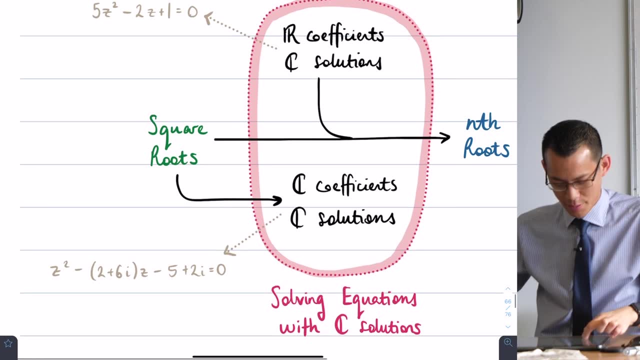 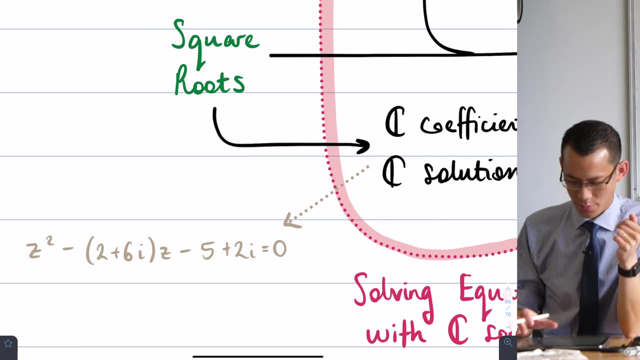 see, here you've got complex coefficients. you're going to get complex solutions. I should point out there is a very, very small family of coefficients that we're going to find that are actually real. They're very strange and unusual and not really the focus of the course, So we're 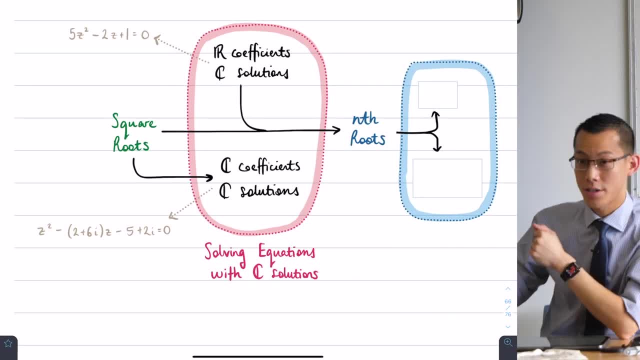 going to do these two examples shortly together. but before we leave off this, I do want to anticipate. next week we're going to focus on nth roots and we're going to do it in two kind of halves right. The first is we're going to look at the nth roots of a special complex number called. 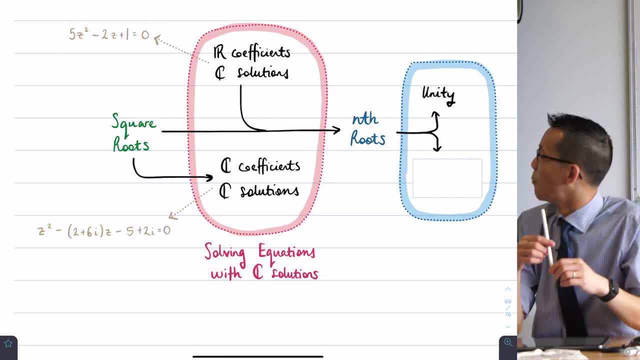 unity. We love giving fancy names to things. right, You'll be able to see that we're going to be less impressed by what unity is once we actually get there, but it is a special number nonetheless. And then, once we go from there, we're going to have a look at: well, what if we?